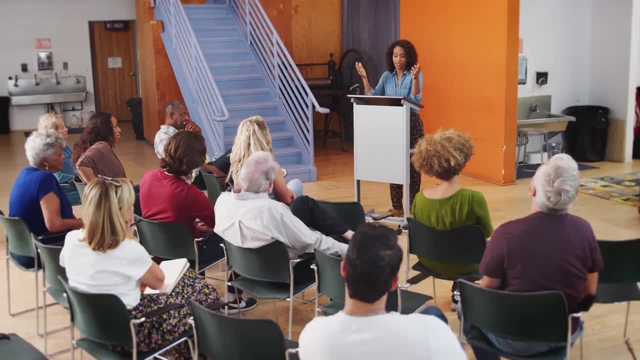 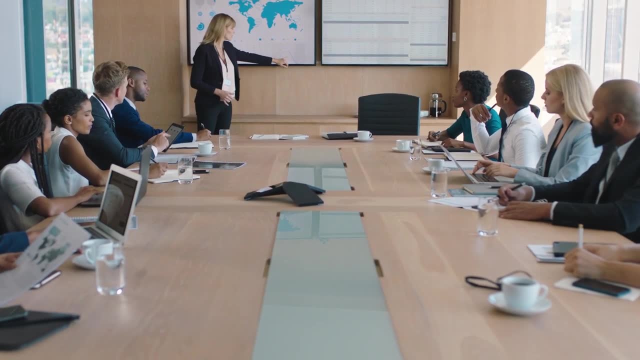 Information is not synced across planners, developers and city leaders, causing the urban planning process to take a lot more time, effort and money, And, unfortunately, these workflows are often limited to 2D maps, lacking the ability to visualize and understand the city at the street level. 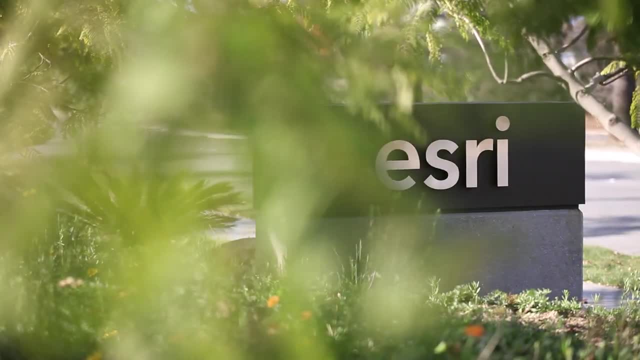 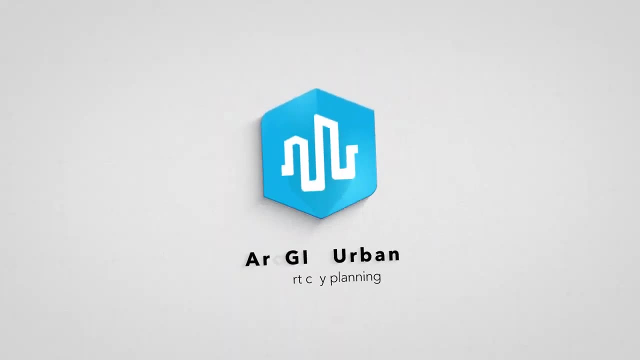 which can help make smarter planning decisions. That's why Esri has created a 3D web application that streamlines all these workflows for a more efficient urban planning process. ArcGIS Urban is a 3D web experience that orchestrates urban development and planning workflows. 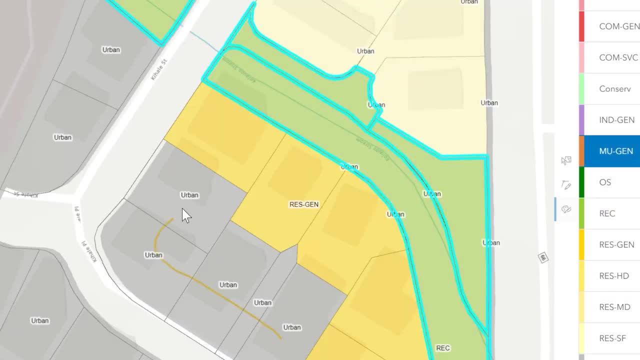 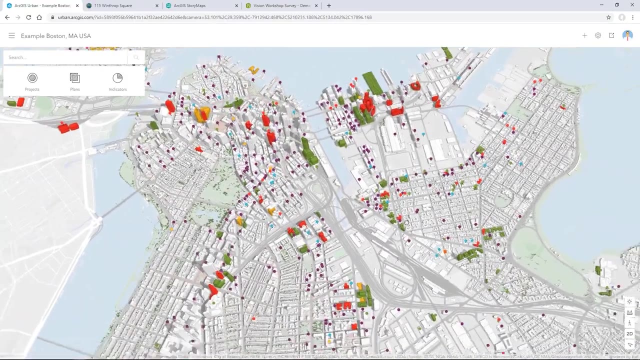 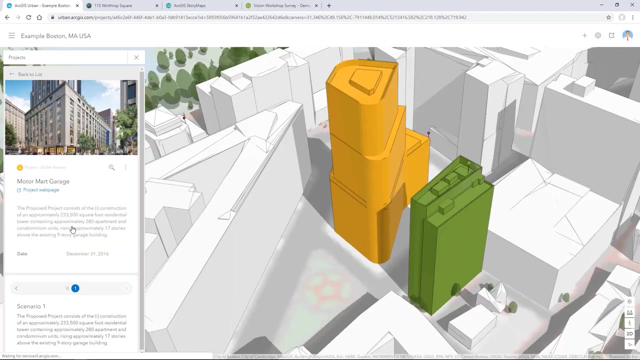 by streamlining the creation and sharing of data, land use and zoning plans. alongside the review of proposed development projects, This helps all organizations involved in the planning lifecycle to coordinate efforts more efficiently, using ArcGIS Urban's single city-wide view, By distinguishing projects by size, type and even development status. 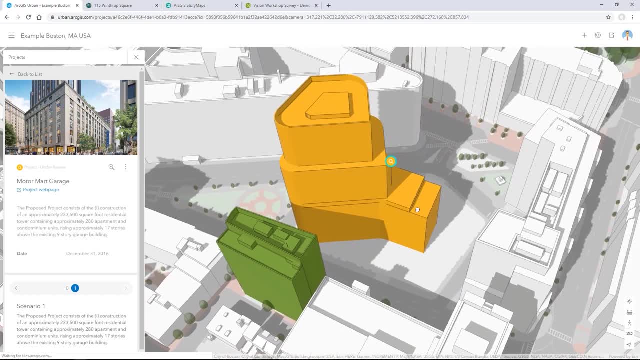 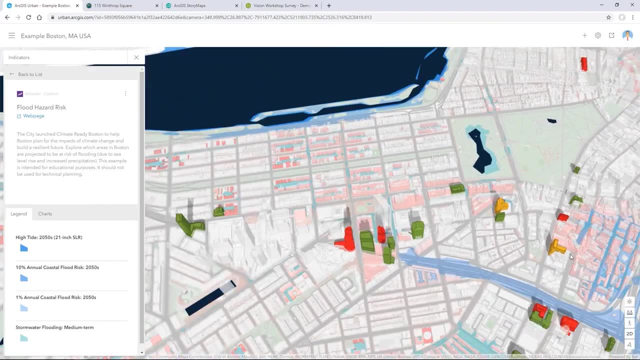 Esri's smart city planning tool makes it easier to track building development and infrastructure. Planners can see where projects are, understand the proposal in its spatial context and explore important indicators related to environmental constraints. ArcGIS Urban can support your local regulations. 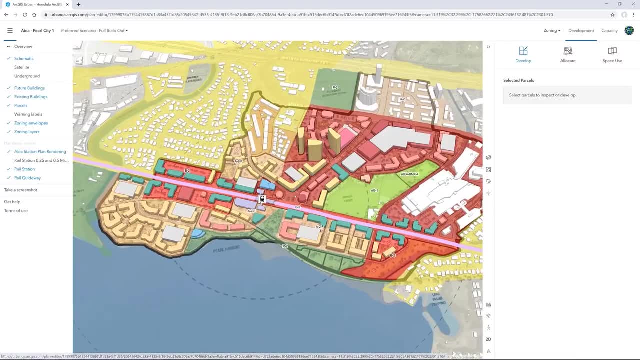 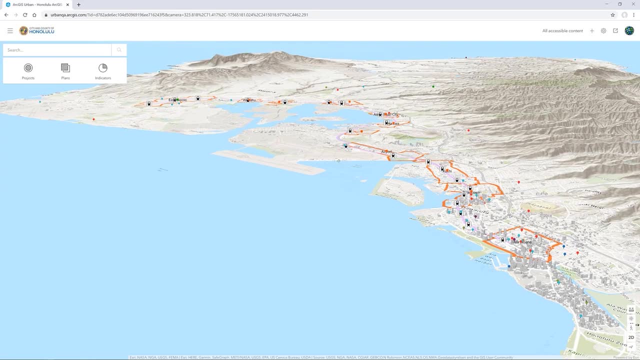 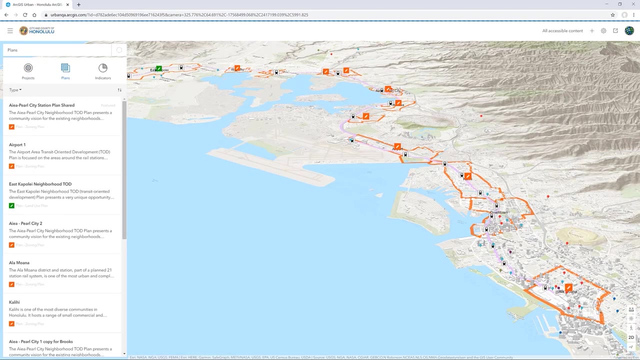 enabling planners to author land use and zoning scenarios in a 3D context and provide downstream reporting for key capacity metrics like household units, trip generation, parking and emissions. ArcGIS Urban provides an interactive overview to coordinate the planning process, improving data consistency and the organization of planning teams. 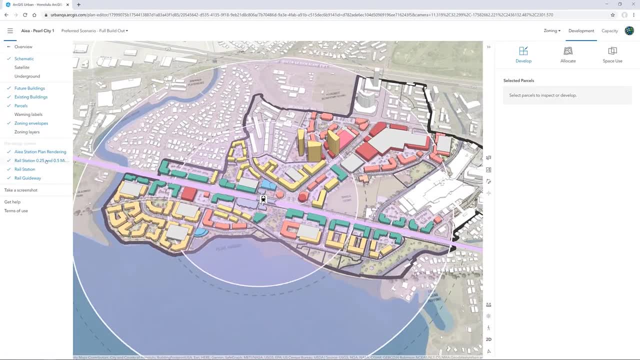 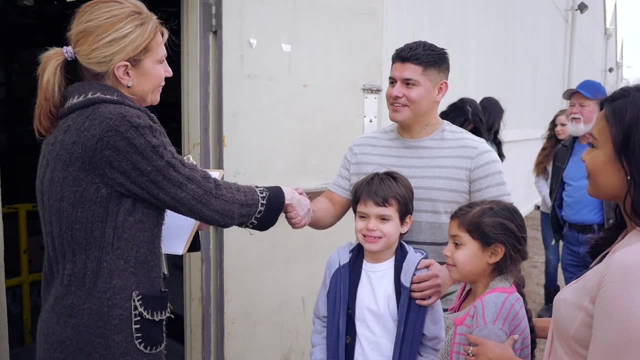 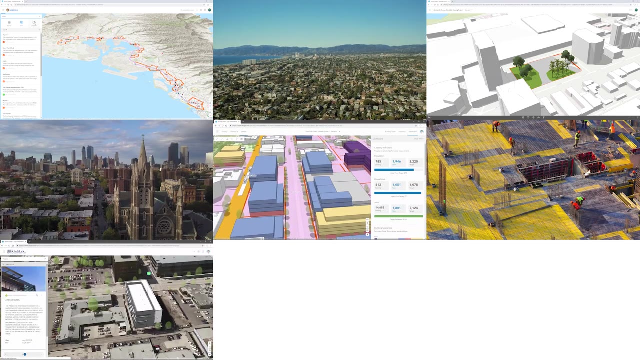 Planners can easily move traditional policymaking towards a more analytical and scenario-driven process, share and review incoming development proposals with stakeholders and the community for valuable feedback and measure performance indicators, city-wide accounting for individual plans and projects. ArcGIS Urban helps organize city and regional planning initiatives for a more holistic urban planning process. 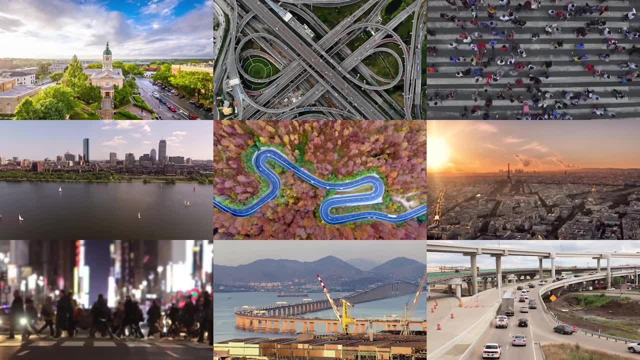 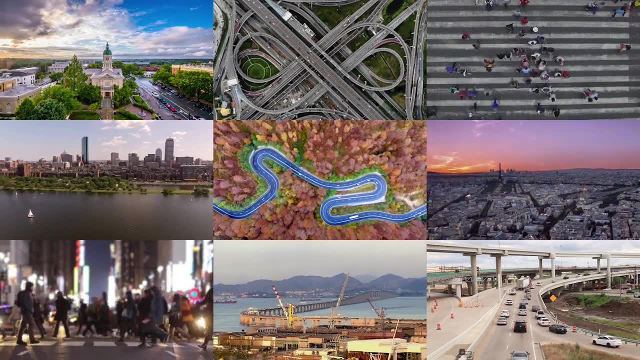 so that planning teams can streamline collaboration with local developer and architecture firms and deliver community engagement by providing a way for citizens to review and comment on plans and projects over the web. Become more proactive and less reactive in your planning process. Simplify project collaboration across internal agencies.